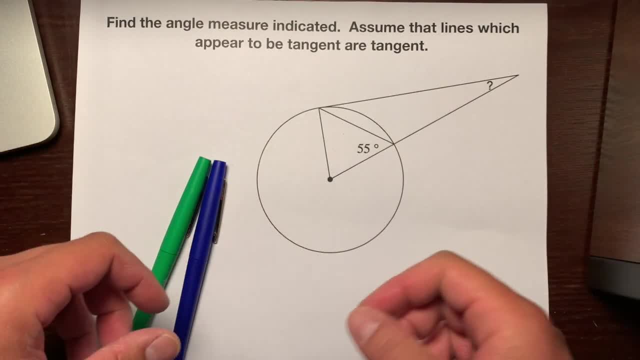 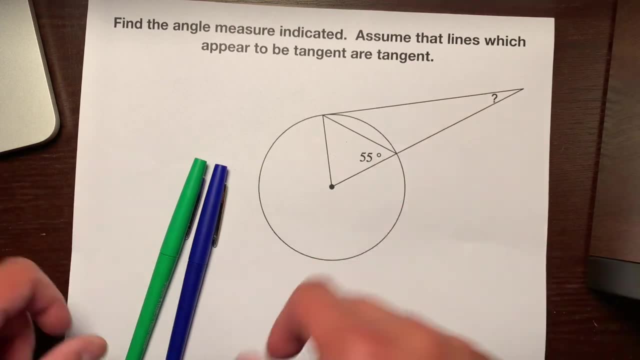 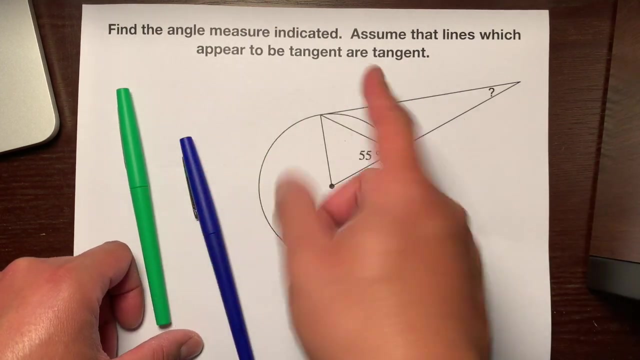 Hello, this is Mr Kenyon Nola and I'm going to help you find the angle measure indicated. So here's the indicated angle and I'm going to help you find the measure of this with two pens, because I'm going to show you two different ways of how to do this problem. So first thing is let's read: 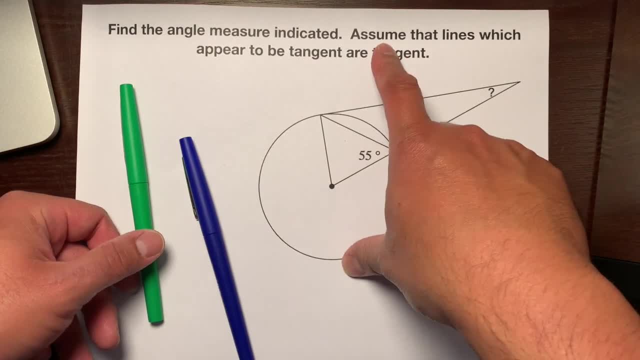 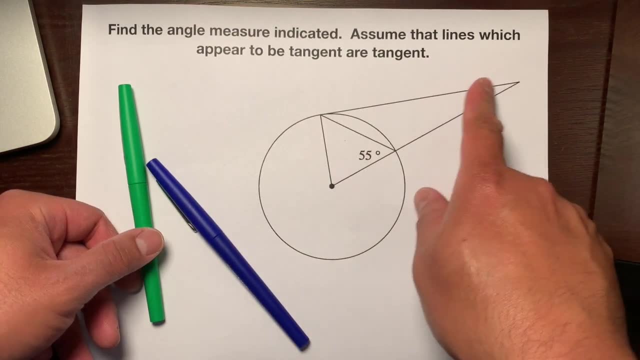 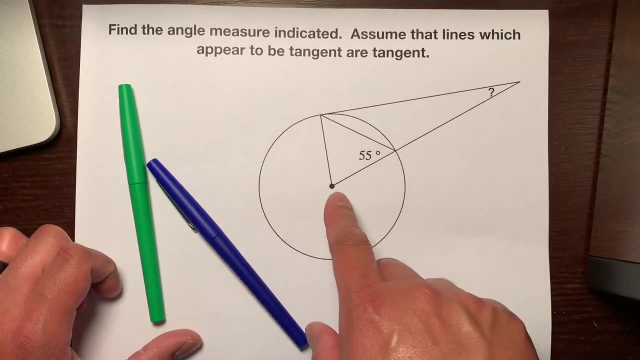 the rest of the instructions Assume that lines which appear to be tangent are tangent. So this line right here appears to be tangent because it appears to touch the circle at exactly one point right there, And here's a radius that touches that point of tangency right there. So if you 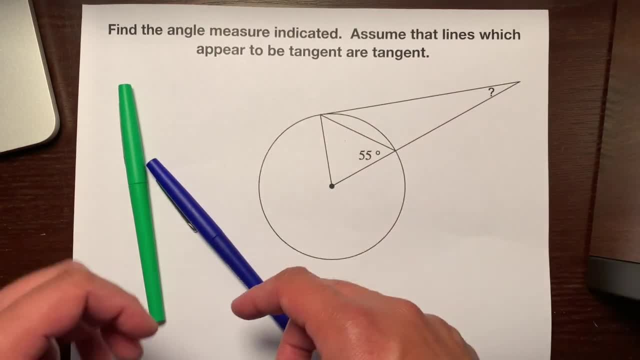 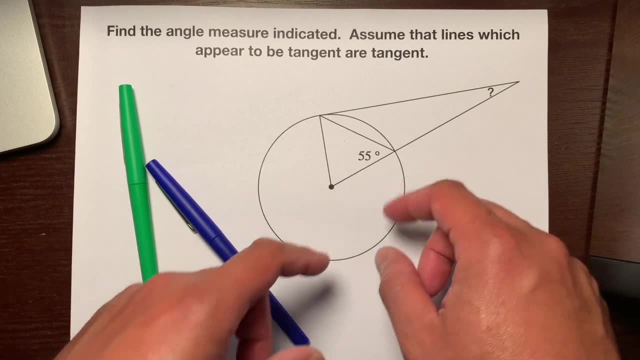 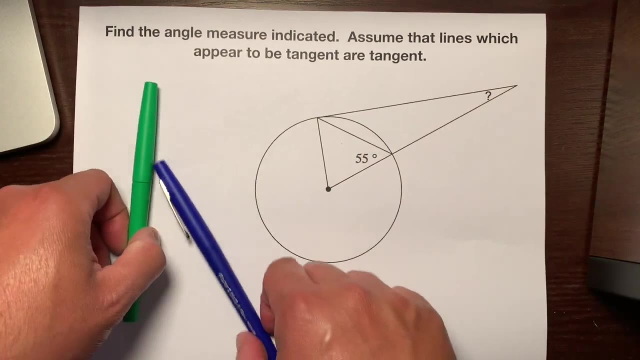 guys remember, if you guys watched the previous video where it teaches you about radii and tangent lines, and when a radius and a tangent line intersect, at the point of tangency, they make perpendicular lines, And perpendicular lines are: they make 90 degree angles. So because this, 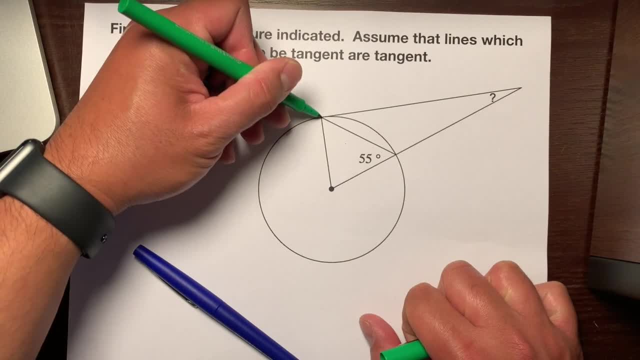 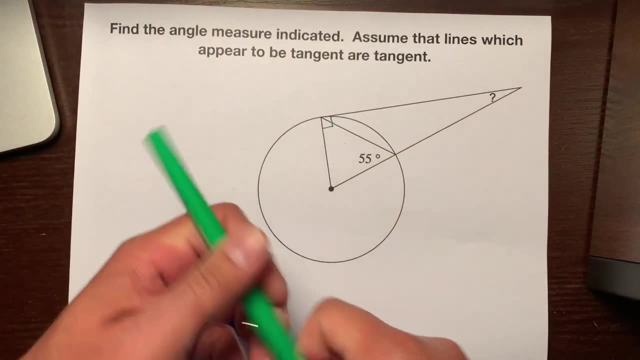 line that appears to be tangent really is tangent and here's a radius that intersect at this point of tangency. that means this angle is 90 degrees because they are perpendicular. So if you didn't watch the previous video, watch it. It's super interesting. I don't know if it's that interesting. 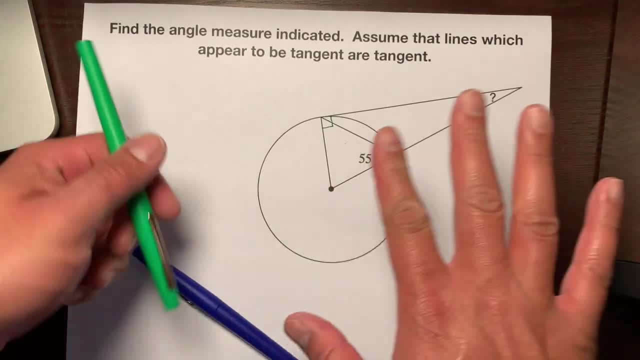 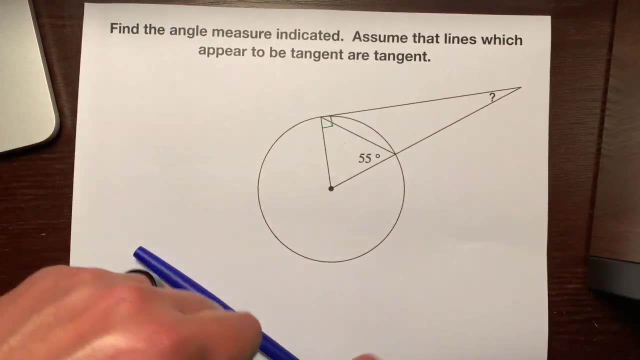 but I think it's interesting. Maybe not super interesting, Eh, it's kind of interesting, It's interesting, Okay. so there's that. So here's the first way of doing this problem. So we have two radii. Okay, radii is plural for radius, And if you 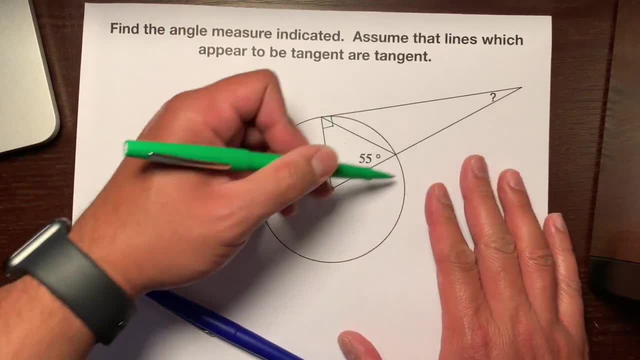 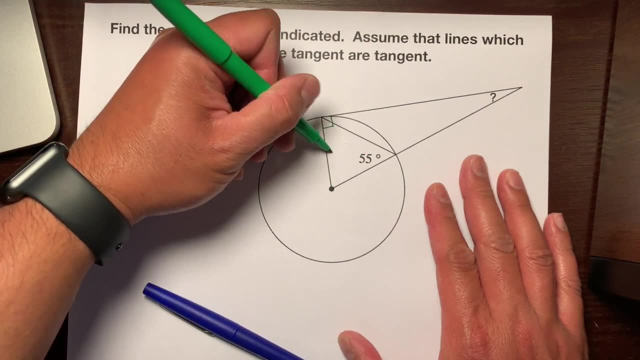 guys remember, all the radii in the same circle are all congruent. So that means this side, this radius and this radius are congruent to each other. So I'm going to put a tick mark and a tick mark right here. And so look at this, We have this little triangle. 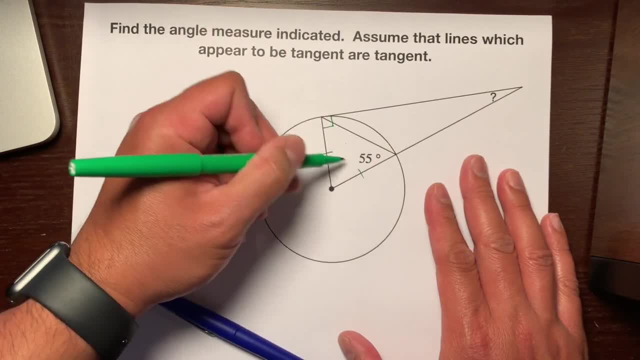 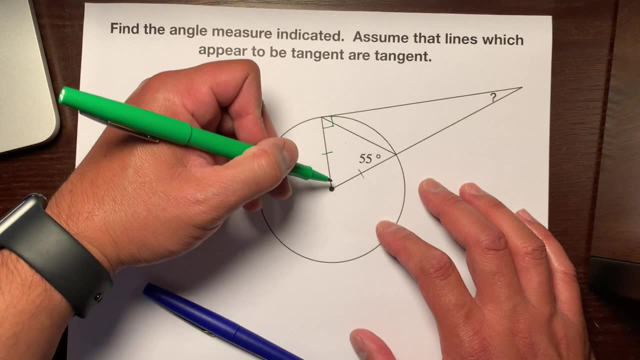 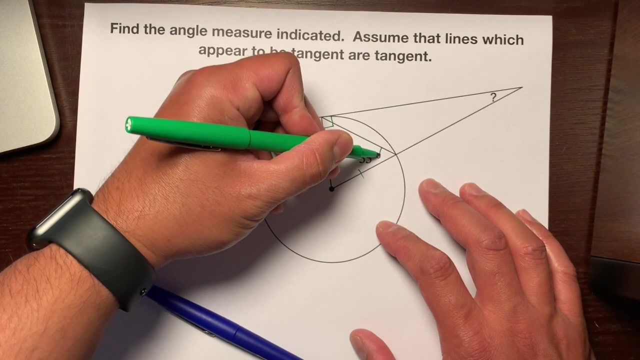 Right here, with the tick mark here and here. If these two sides are congruent, that means that this triangle is isosceles. And what kind of angles do isosceles triangles have? What is that? What did you say? Yes, base angles. So that means that this angle right here is a. 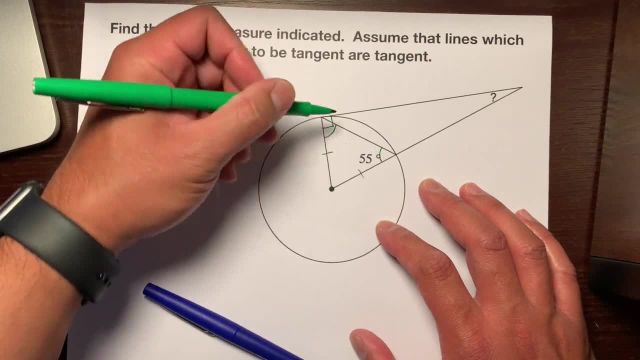 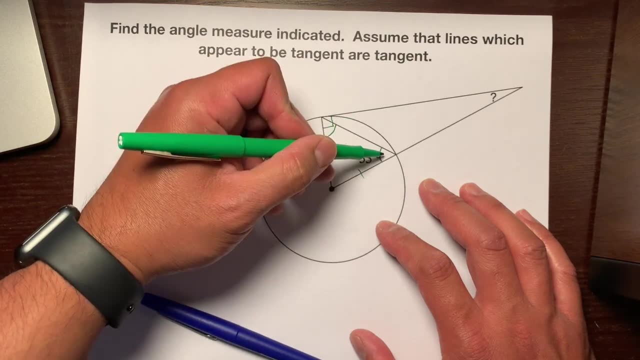 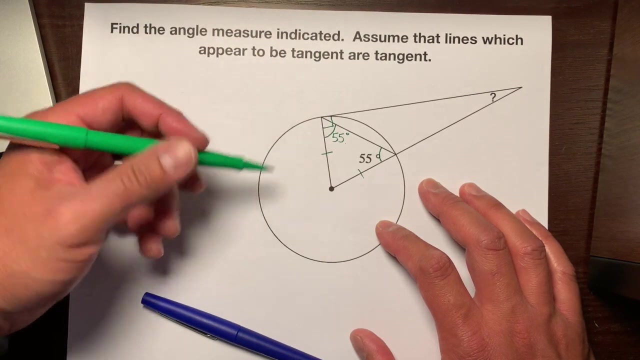 base angle to this, And that means these base angles are congruent. So not only do isosceles triangles have two congruent sides, they have two congruent base angles. So if this angle is 55,, 55 degrees, then this angle is 55 degrees. So there's that, And then what we're going to do. 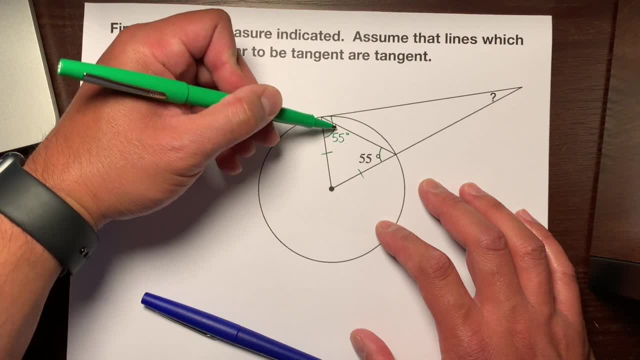 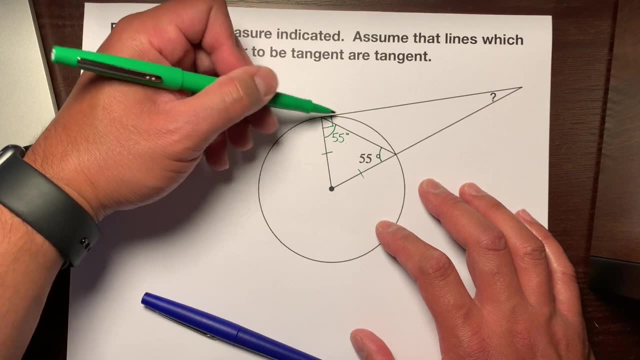 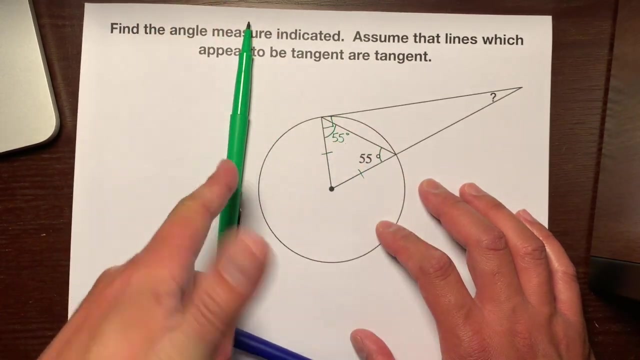 next is we're going to use this right angle right here. So this angle right here is just 55 degrees, But this is a right angle. So that means these two angles add up to 90.. What kind of angles add up to 90?? Well, let's use this little pointer right here And this. Oh hey, this is a nice pen. 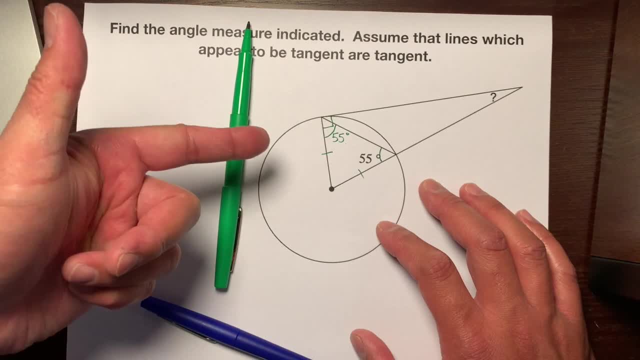 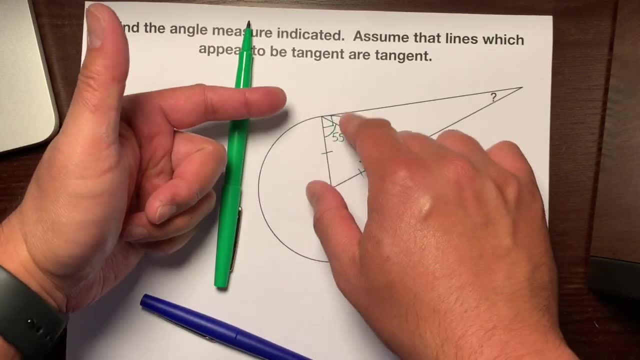 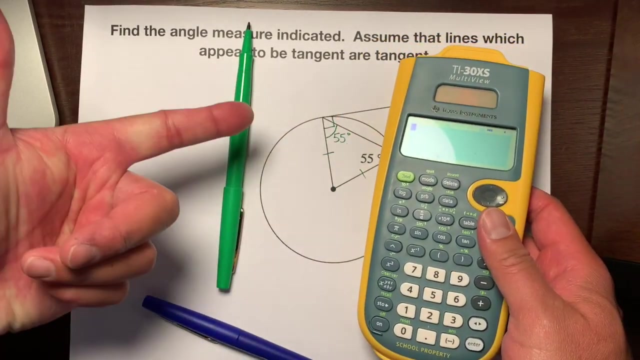 I just complimented this green pen, saying it's a nice green pen. If I turn my hand to the side, it makes a right angle, 90 degree angle. So that means that these two angles add up to make a right angle, or they add up to make 90 degree angles. So complimentary, Hey, yeah, Hey you. 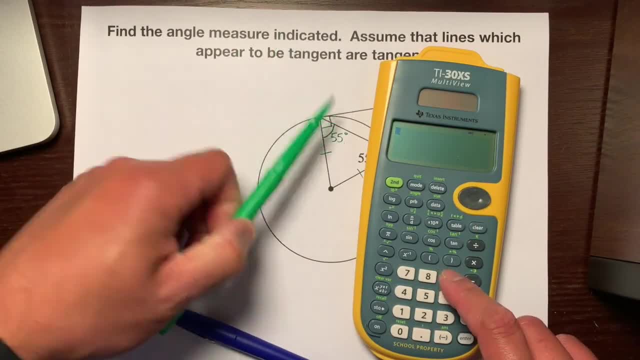 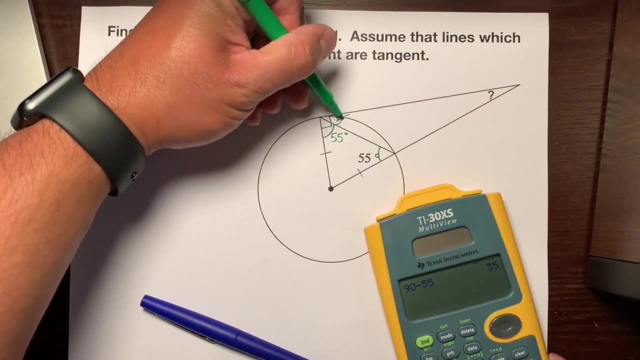 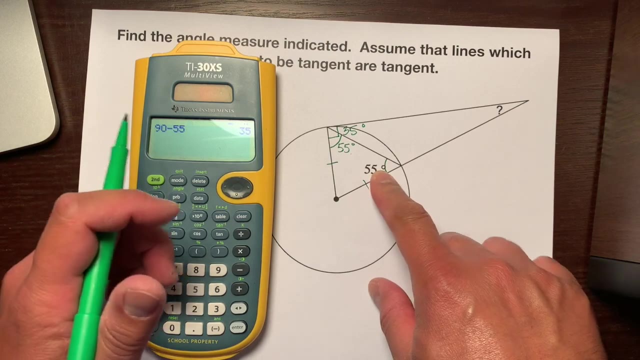 look nice today. So to find this angle, we're going to take our calculator, take the 90 and subtract 55 from it. That makes this angle 35 degrees. Okay, Next thing is we're going to use this 55. And that means this 55 and this right here. 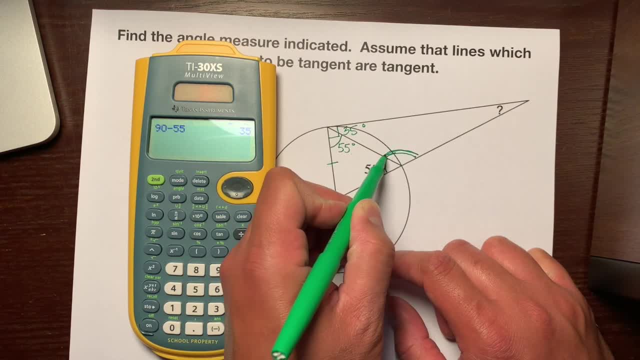 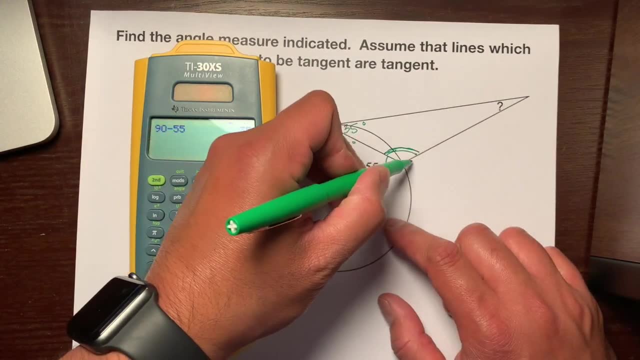 this angle. right here. I'm going to put two arcs to make sure that we don't. we don't think that these two angles are congruent, But these two angles make this straight line. So these two angles add up to 180 degrees and two angles that add up to 180 degrees. 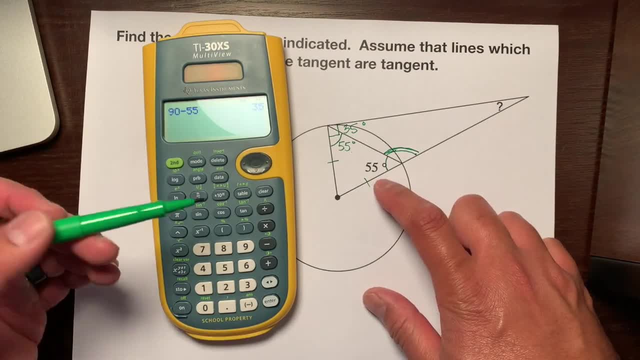 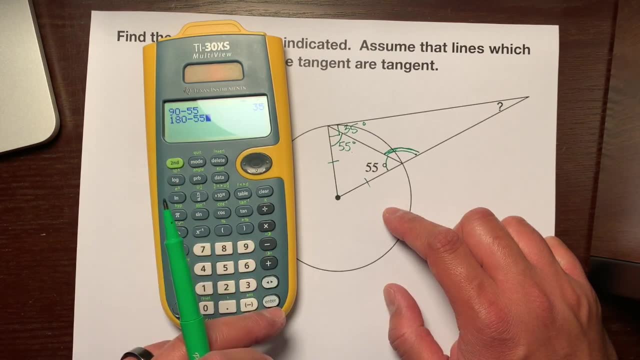 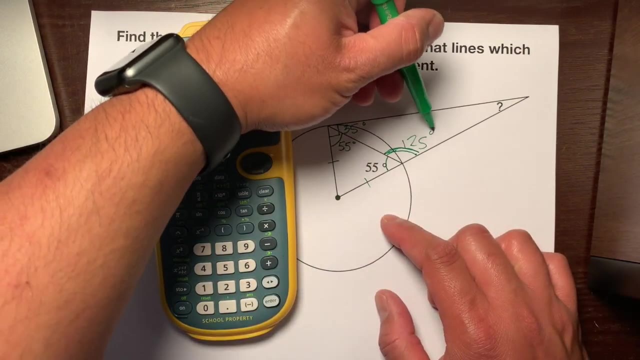 supplementary. So, uh, what we're going to do is take our calculator again: instead of 90, we're going to, we're going to type in 180 and subtract 55. So this, it's supplement: 55 supplements is 125 degrees. So now we're going to focus on this triangle right here. 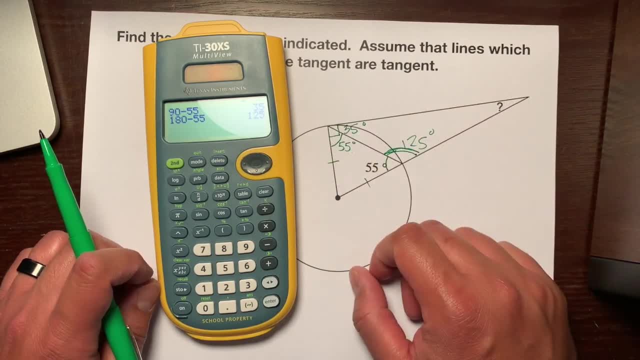 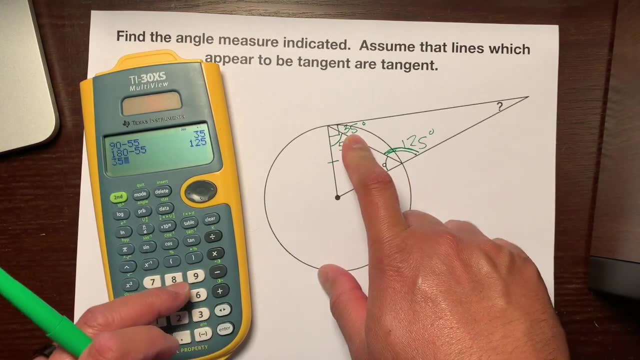 and all three angles. because of the triangle, some theorem, all three angles add up to a 180 degrees. So we're going to take this 35 and add one 25 to it, And that's 160. And we're going. 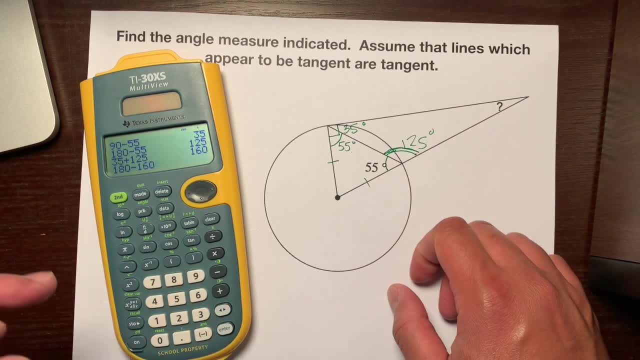 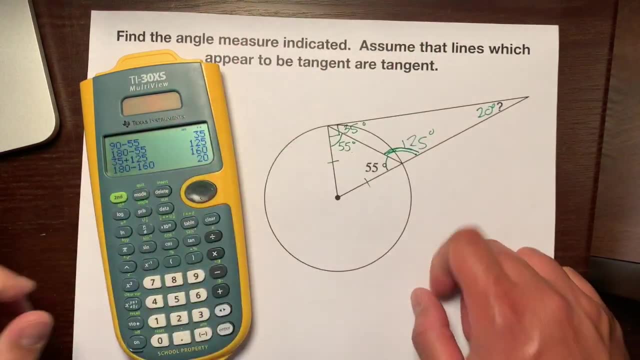 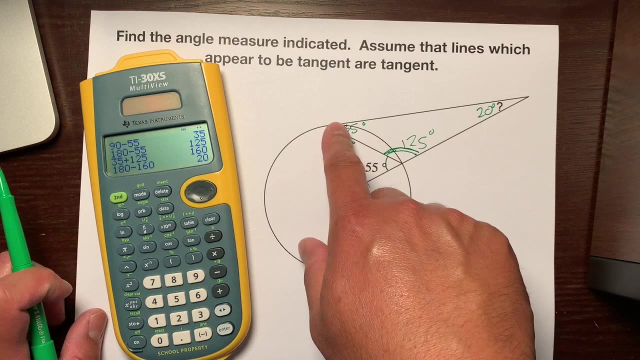 to take 180 and take away 160 from it And that makes the indicated angle 20 degrees. So that's the first way of figuring out this indicated angle. uh, tangent line radius. They are perpendicular, So they make 90 degree angles. Both radii are congruent, So they make a. 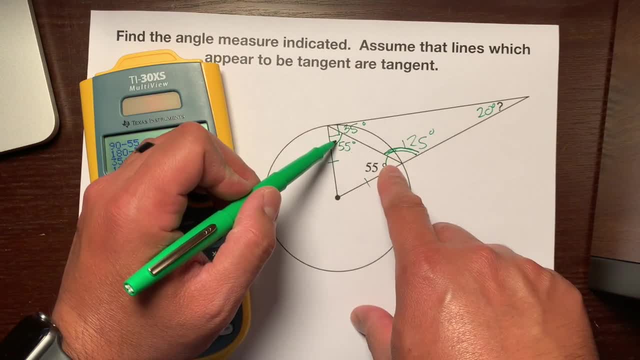 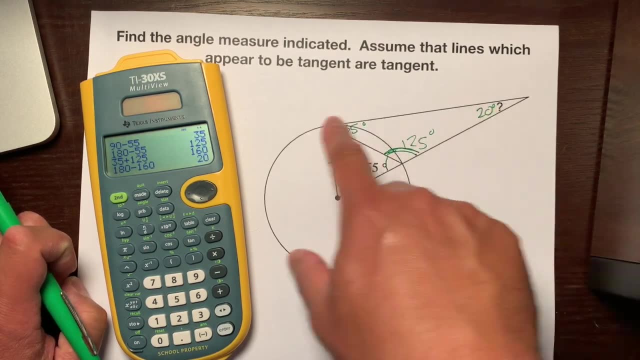 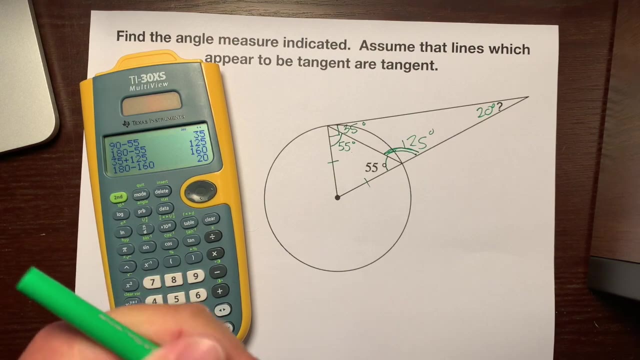 isosceles triangle. Isosceles triangles have base angles. for this base angle 55.. Uh, these two are complimentary, These two are supplementary triangle. some theorem, 20 degrees. That's a lot of vocabulary, I know, Uh, but uh, you sound cool while you're saying. 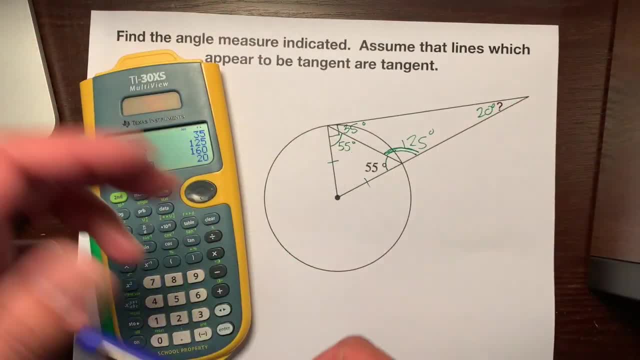 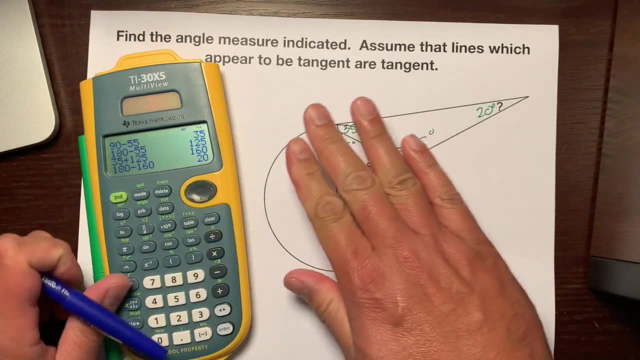 all this stuff, If you'd say correctly. I don't know if you sound cool, but whatever, Okay. So, uh, the next way of doing this, I'm going to take my blue pen and let's pretend all of the stuff that. 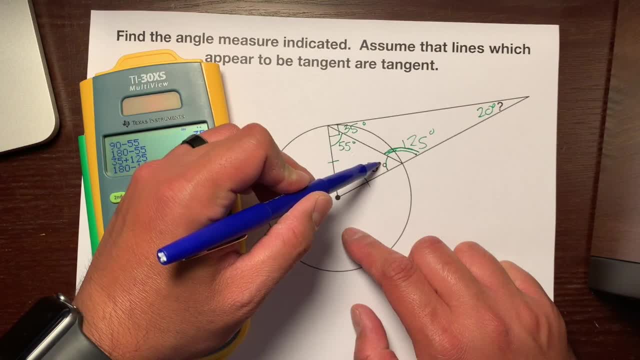 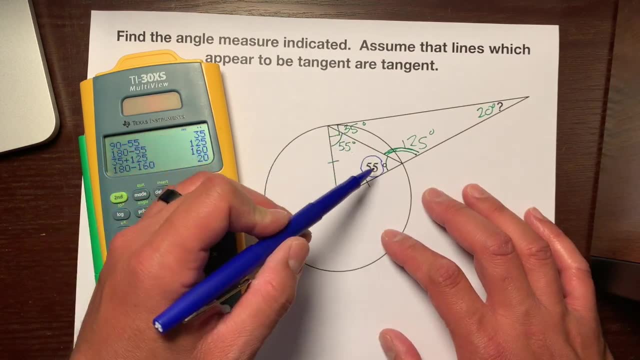 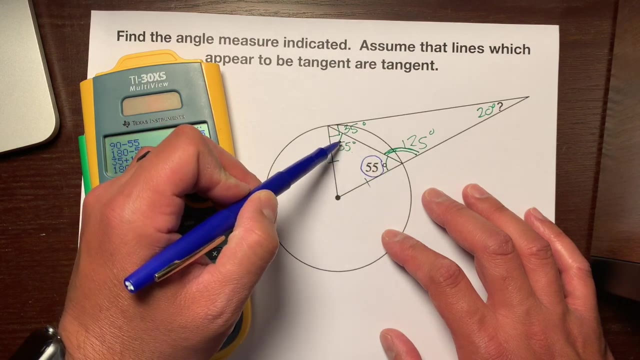 isn't here. The only thing that they gave us was this: 55 degrees right here. Okay, So, uh, we're going to use the same fact that this is an isosceles triangle is a radiate. uh, the two radii are congruent. So this is isosceles And we have this base. 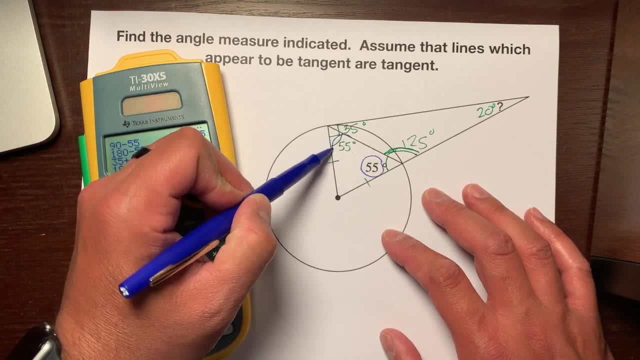 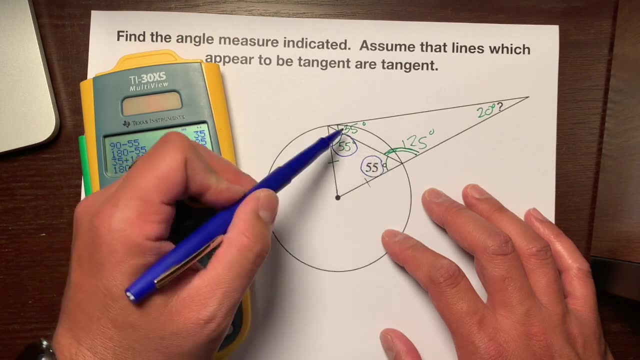 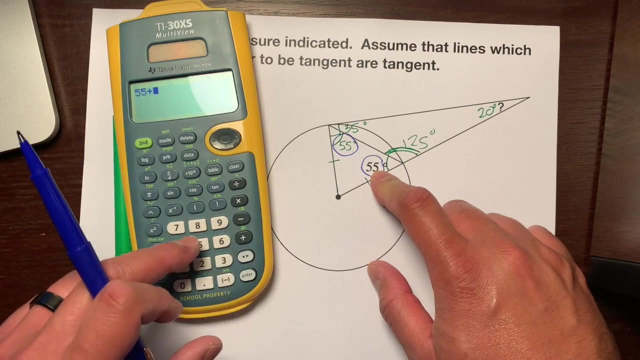 angle right here, which is congruent, So this is also 55 degrees, And we want to find this vertex angle right here. So, uh, with this little triangle right here, all three angles up to 180 degrees because of the triangle sum theorem. so i'm going to take this 55, add the other. 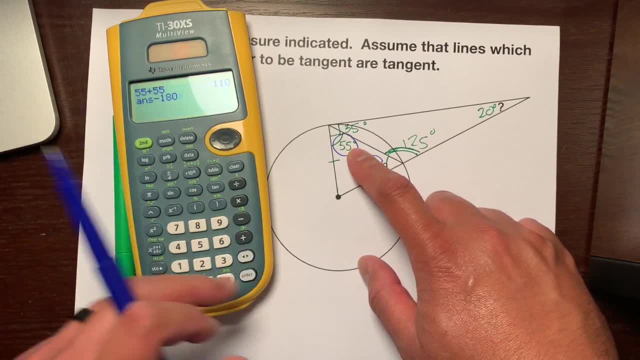 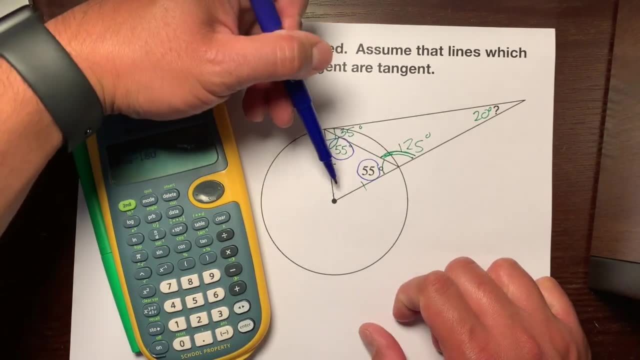 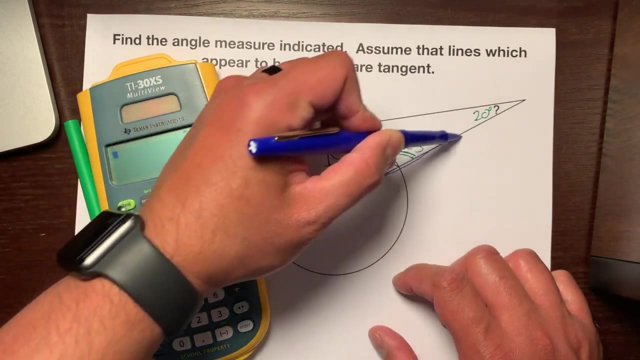 55 and subtract it from 180. uh, it shouldn't be negative 70, it should be positive 70, because 70 plus 55 plus 55 equals 180.. so this is 70 degrees, and now we're going to focus on this big triangle. 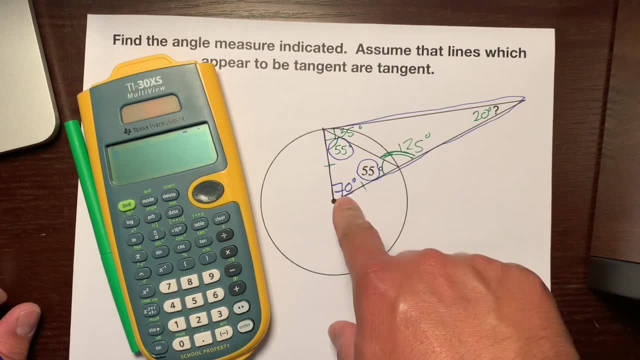 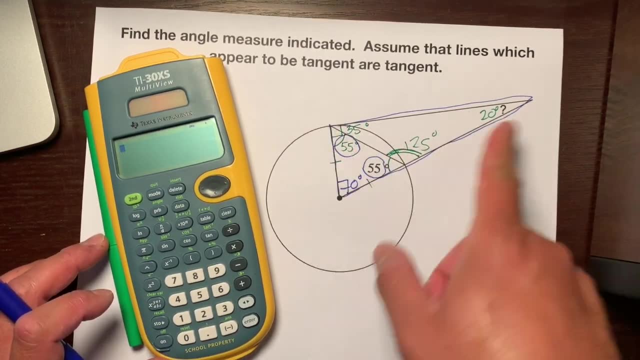 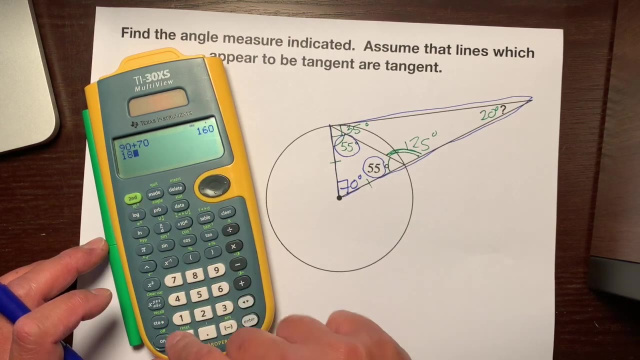 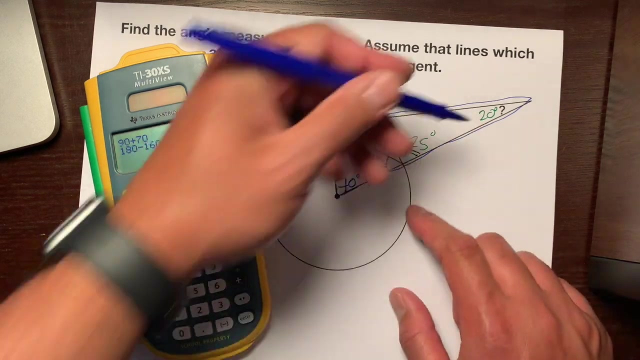 right here. and since this is 70 degrees and this entire angle is 90 degrees, okay, so we're going to use a triangle sum theorem: 90 plus 70 is 160, and we're going to take 180 and take away 160 and will you look at that? you get the exact same answer: 20 degrees. i want to write it in.